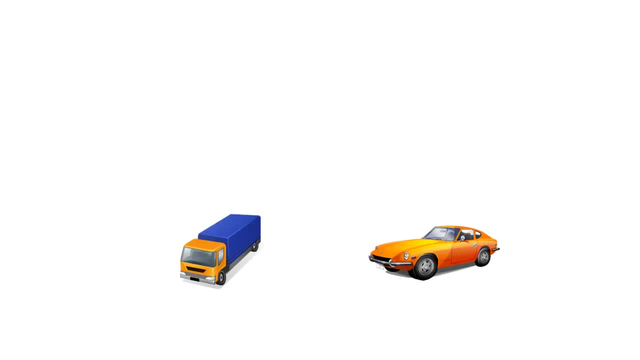 example, consider cars and trucks. They're different, but they're both vehicles, So you could say that a vehicle is a higher level description or an abstraction of a car or a truck. Now consider a dog. If we take a step back, we could say that our dog is an. 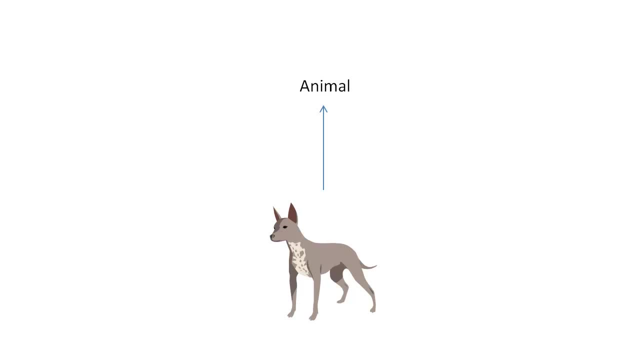 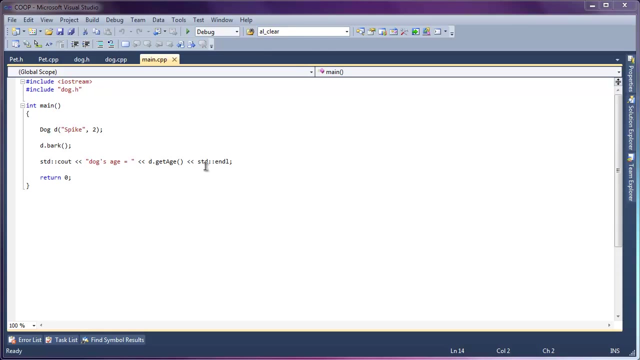 animal. However, this might be a little too abstract for our purposes, so we're going to use a slightly lower level of abstraction: a pet. So you'll see that I essentially have what we left off with in the previous video, except I've added a petcpp and a peth file, And this is where we're going to implement our 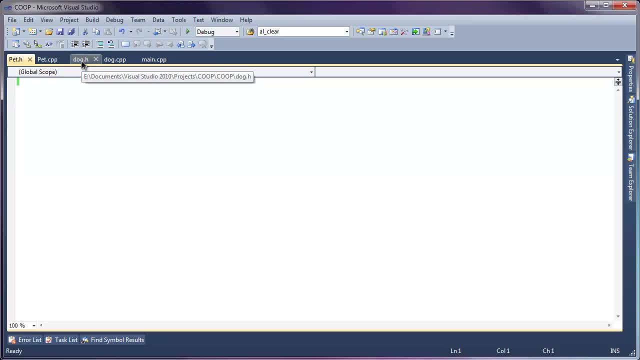 pet class And naturally our pet class is going to have a very similar structure to our dog because, well, our dog is a lower level description of our dog, So we're going to 여기 throw in the name of our dog and print out our dog. so we're going to create 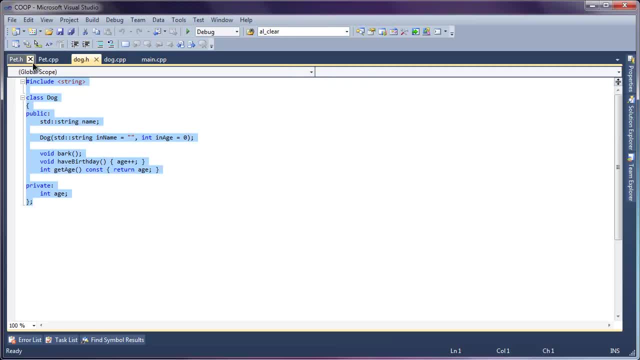 a unique, So we're going to pass it over 소개 dogtype, so our dog might be. We could also call our dog doggie, So we could include the subject under a donnec ração that we just created and then just describe in there what that dog is like And 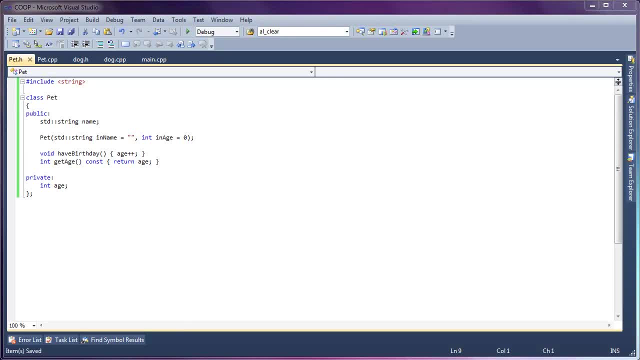 we can also define a tentar, which is your dog, So I can change the city and we can ahead and complete the implementation of our pet class. It's fairly similar to the way that we did our dog. We don't have a bark method, so I'm just going to copy and paste. 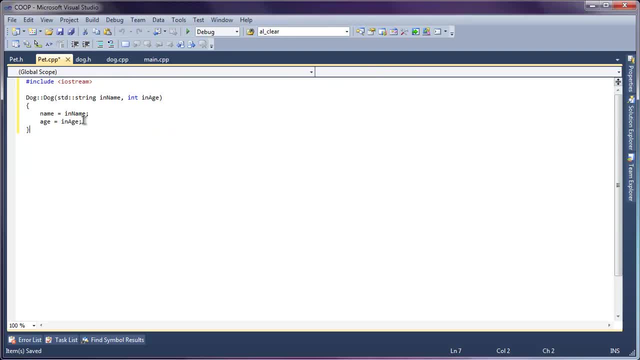 this top part, go in here, and we can't forget to include our pet header file, and we have to rename the constructor and specify the proper scope. So there we go. we have a pet class, And what exactly do we do with this now? Well, we could use it just like we use the dog class. 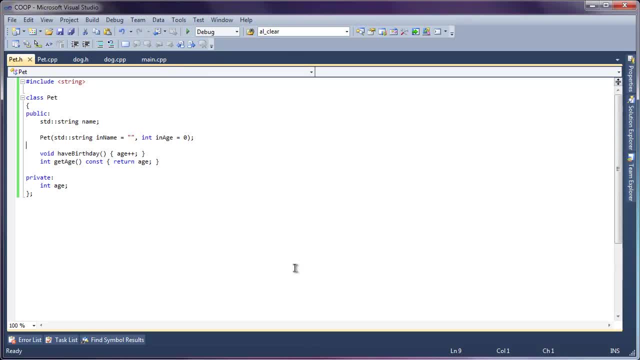 right now, but that doesn't really make our job any easier than before. Like I mentioned earlier, though, a dog is just a specific type of pet. Naturally, you could say that a dog inherits the attributes of a pet, and this is arguably the most important aspect. 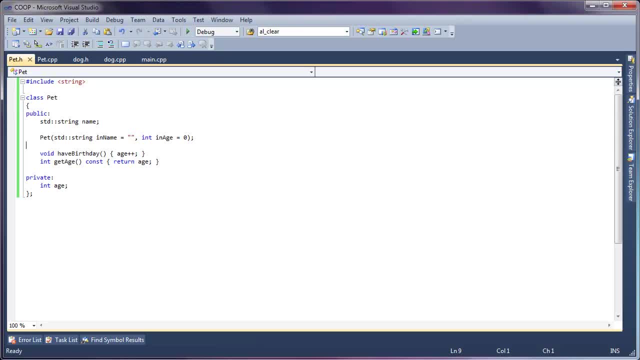 of object-oriented programming inheritance. Now, because we've already written this code here in our pet class and we've defined a lot of this in our pet class, what we can do is we can just inherit that from our pet class, So I'm going to go ahead and delete. 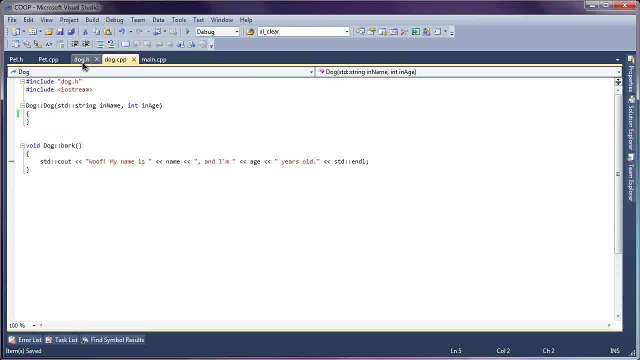 some of the implementation here for our dog's constructor, and I'm going to delete a lot of our dog's definition. And the reason I'm doing this is because this stuff is already defined here in our pet class, so there's no use defining it a second time Now if we want to inherit these attributes. 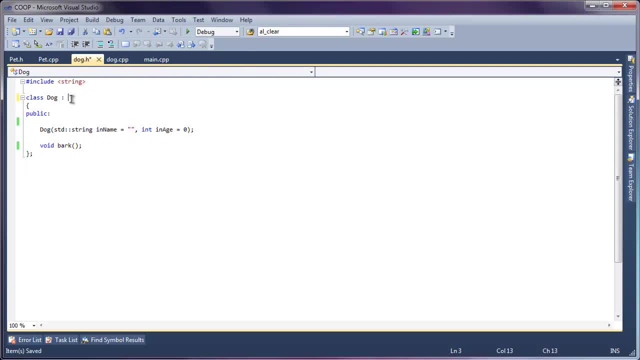 and methods. it's really simple. What we do is we just use a colon, which is basically saying that we're extending or we are inheriting our pet class And we can't forget to include our pet's header file. So again, this is how we inherit. 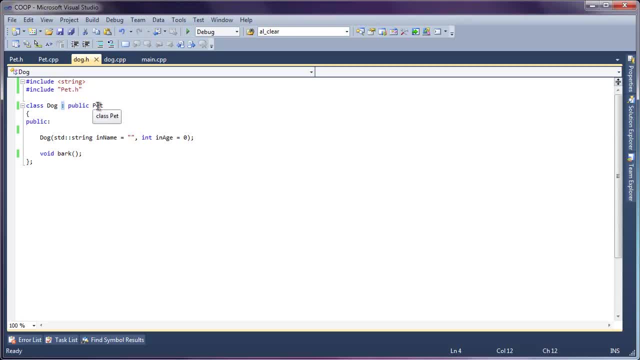 another class. We use the colon to specify that we're inheriting a pet, and I'll talk about this public in a later video. but you know, just use that for now. And in order for this to work, what we're going to have to do is we're going to have 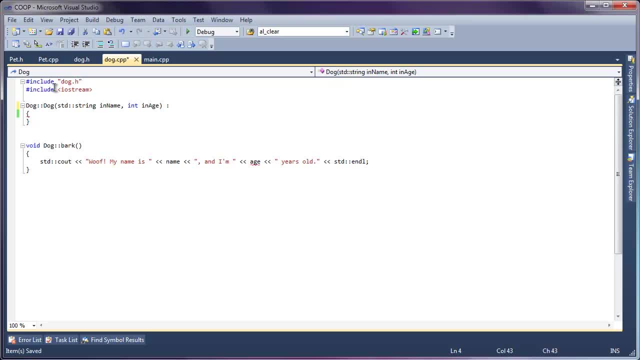 to pass some values from our dog's constructor into our pet's constructor, because this is the function we want to call And in order to do that, we use the colon once again and we simply call the pet's constructor with these values that were passed in to our dog's. 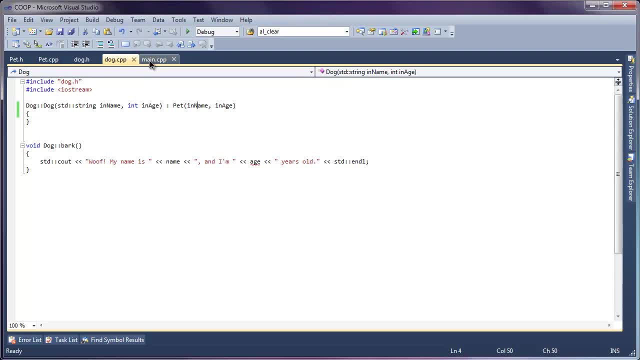 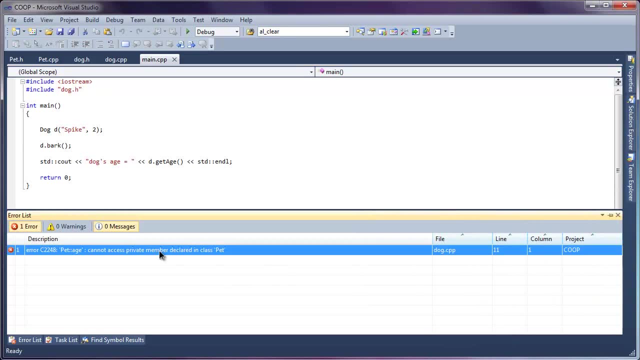 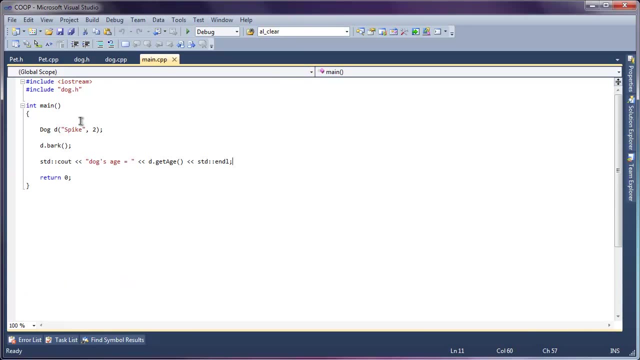 constructor And you'll notice that if we try running this we get an error And I guess the error says that we can't access a private member declared in class pet, which is the age. You'll notice that it's private and we learned in the previous video that. 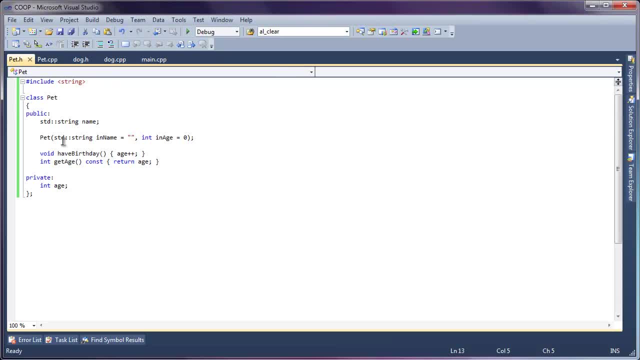 anything that's private can only be accessed from within this class. So if we're trying to access the age from the dog's class, that brings up some issues And to get around this, what we do is we change this access modifier to something else called. 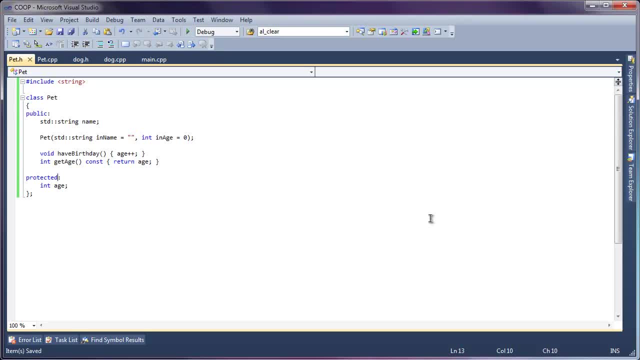 protected, And I suppose you now know that there are three different types of access modifiers, One being public, another is private and the third is protected, And protected is essentially the exact same thing as private, except this will allow any classes that inherit the pet class to access this directly. 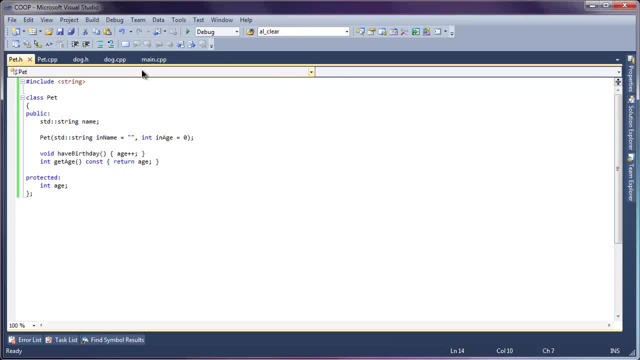 You'll notice that we still wouldn't be able to access this age from outside of any of the inherited classes, say the main function, And we'll go ahead and try running this again And it works just like it did before, which is perfect. 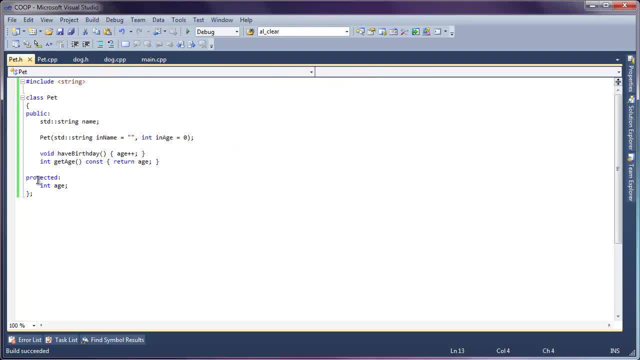 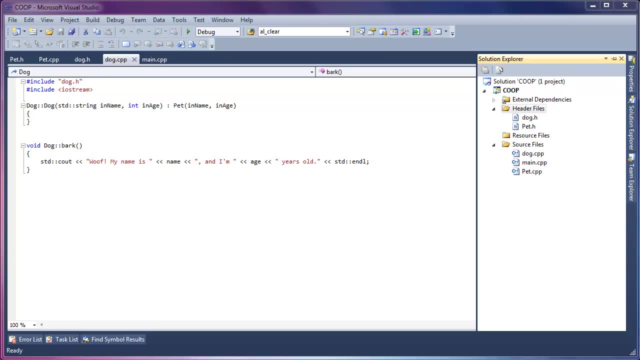 So, again, what we did there was we added this protected keyword so that our dog could access the age directly. Now that we have a base pet class, it becomes really easy to add additional pets. For example, if we wanted to add a cat class and a mouse class, all we have to do is extend. 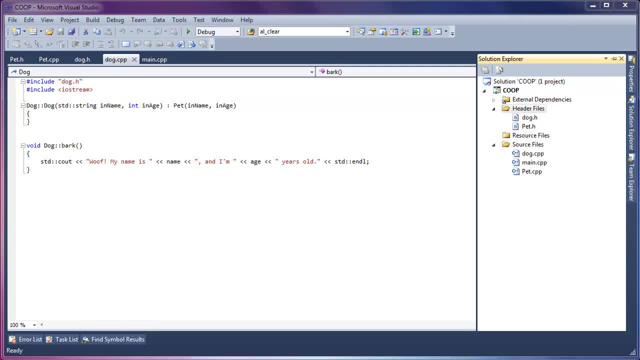 our pet class Without inheritance. if we wanted to do this, we'd have to rewrite many of the functions and methods that we've already implemented, So I'm going to show you this in action by adding a mouse and a cat class. We'll start off by adding a catcpp. 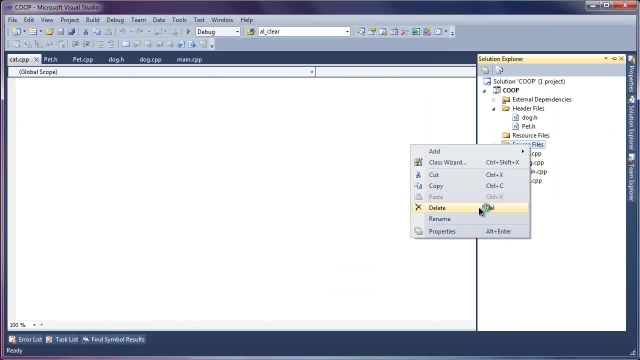 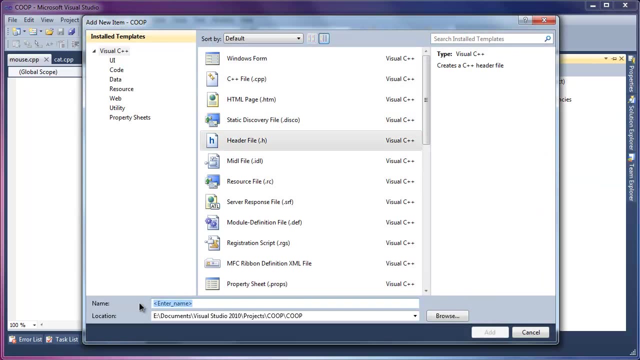 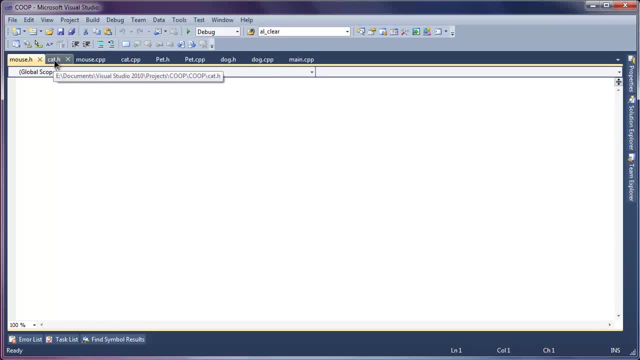 All right. So because our cat and mouse are going to be very similar to our dog in that they're both pets, I can use the dog as a template and simply copy and paste this into our mouse and cat header files. So I'm just copying the dog header information into our mouse. 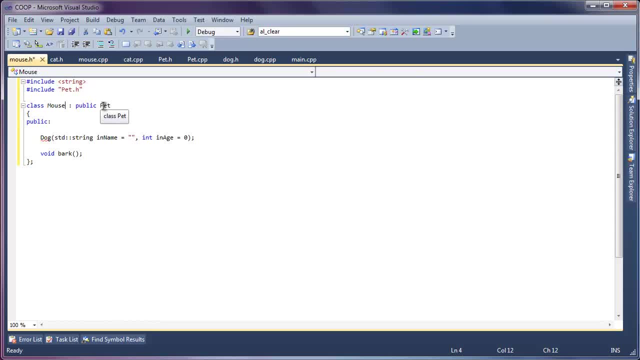 And I'll rename the class mouse. It still extends the pet class And we also need to rename our constructor And we'll change our bark method to something a little more appropriate: squeak. Likewise, we'll go into the cat header file and we'll paste the dog. 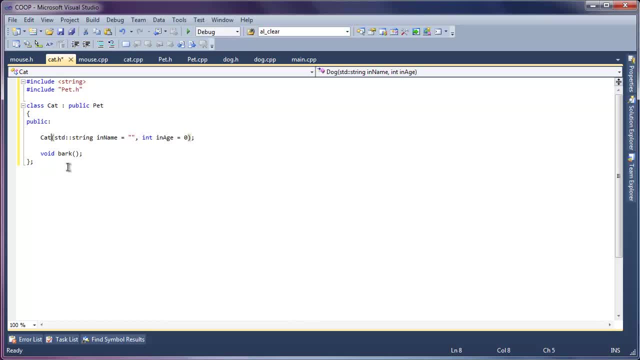 Change the class name to cat, We'll change the constructor to cat And we'll make the cat meow. So now that we have the headers done, we have to complete our implementation And basically what happens when we're extending this pet is that we're gaining access to. 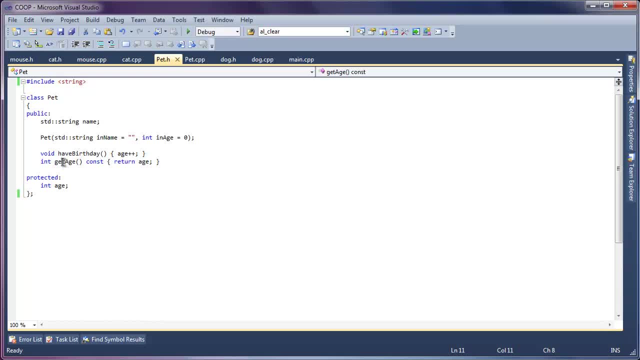 the pet constructor, the have birthday, get age, and our mouse and cat and dog are all inheriting the name and the age members. So all we have to do is we need to specify our name. Okay, And we're going to do that by using our constructor and our bark, or, in the case of a mouse, we'll. 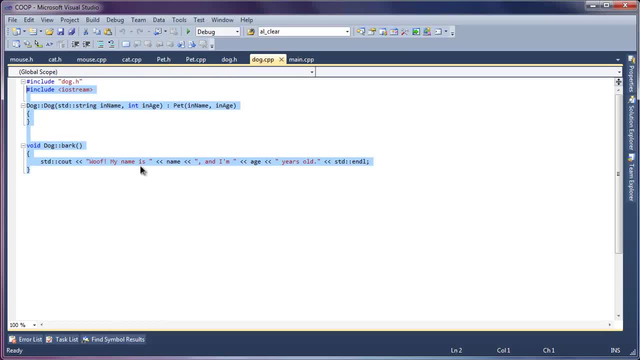 be implementing a squeak And in the case of the cat, we'll be implementing a meow method. So I'm going to start off with the mouse in mousecpp And we have to include our mouse header file, And I- actually I went here and copied the dog once again because I'm using it as a template- 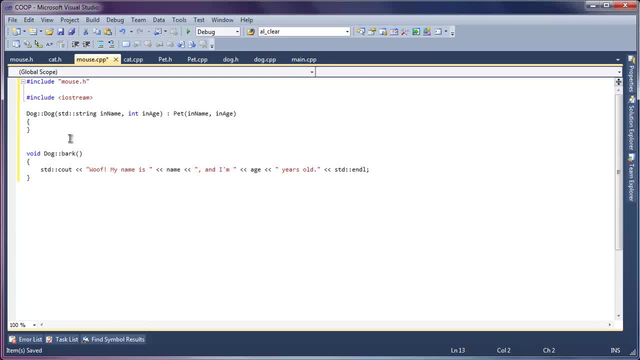 for our other pets, And I'm just going to paste this in here And rename the scope to mouse and the constructor to mouse, And we'll change the scope of our squeak method now and we'll just change a bit of the string that it outputs. 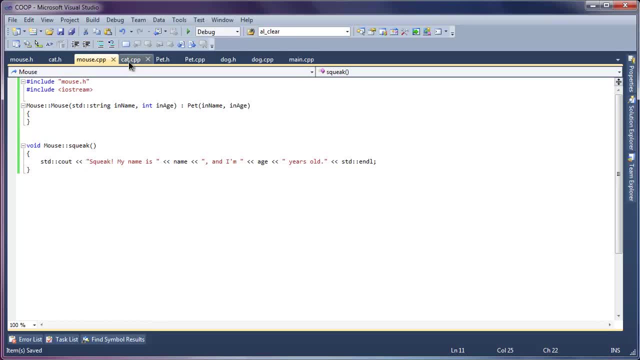 Likewise, I'll do the same in the cat implementation file. Okay, I'll paste in our dog information And I'll include our cat's header file. And, just like I did in the mouse implementation, I just have to rename a few things. 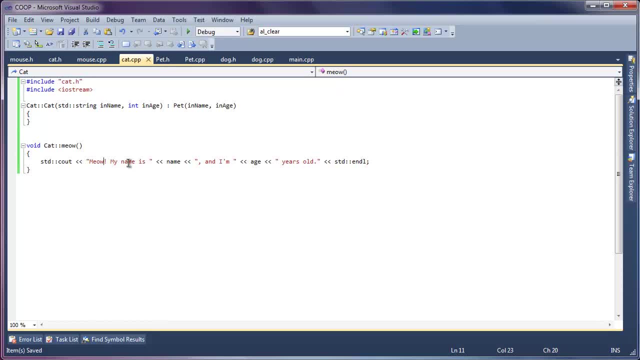 And I'll change the string to meow, my name is, and then it'll output the name and it'll output the cat's age. So if we go to our main function now, we should be able to use these just like we use the dog. 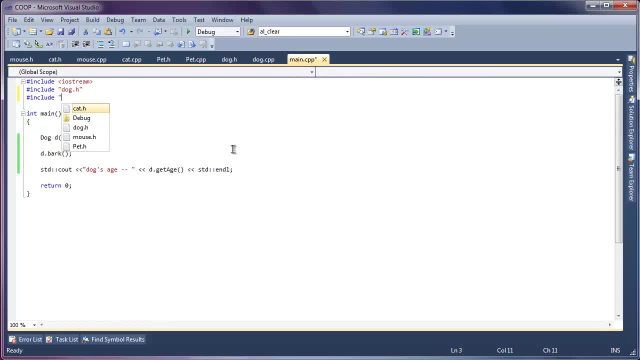 First we have to go ahead and include our mouse header file and our cat header file. This is where the actual definitions of the classes are, And we declare them in a very similar manner: Cat. We'll name the cat Felix And he'll be five years old. 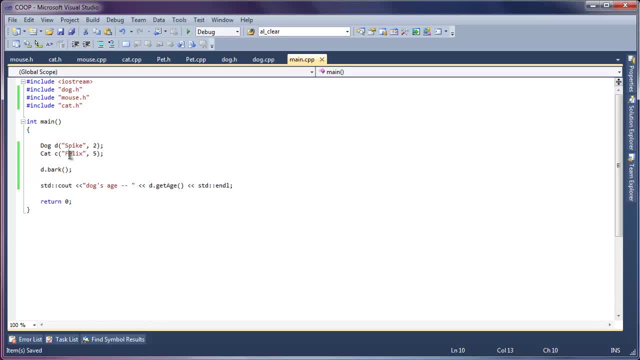 And, as I mentioned before, when we pass these values in, they're going to the cat's constructor And from the cat's constructor we're passing it into the pet constructor, which essentially builds the cat, And we can do the same with the mouse. 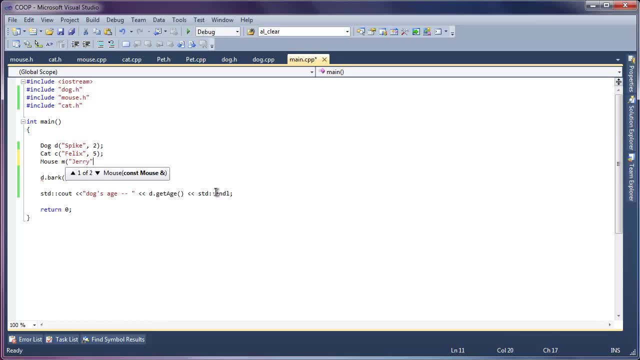 We'll name him Jerry And he'll be one year old And we can do the same thing. We'll go see meow And we'll make our mouse squeak And I'll get rid of this last line here, just for now. 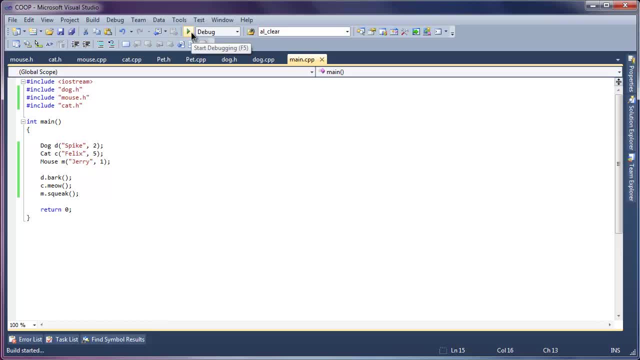 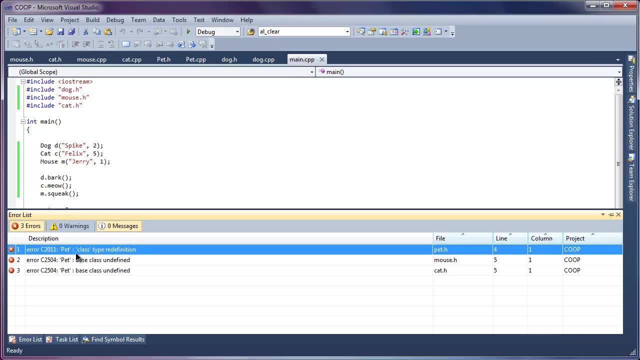 So if we run this, We should get an error. And we do get an error, And the reason for that is that we're redefining our pet class. You might be saying, well, no, we're not. Why are we doing that?